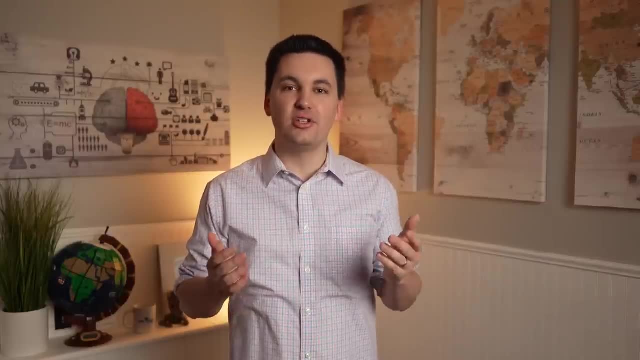 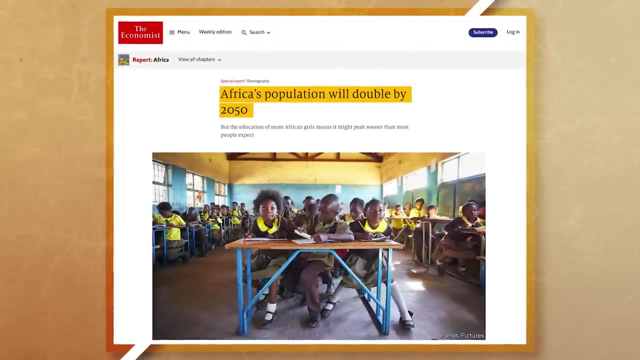 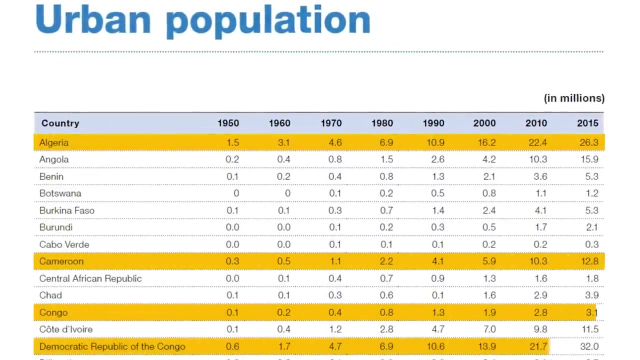 more economically developed countries and less economically developed areas. Africa, for example, is expected to double its population by 2050 and has one of the fastest urban growth rates in the world, which we can see here when looking at the urban population of different African countries from 1950 to 2015.. 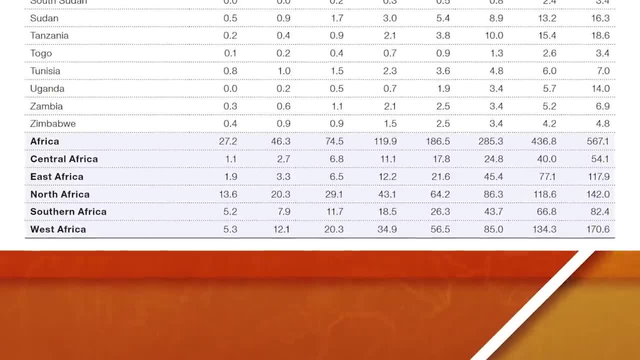 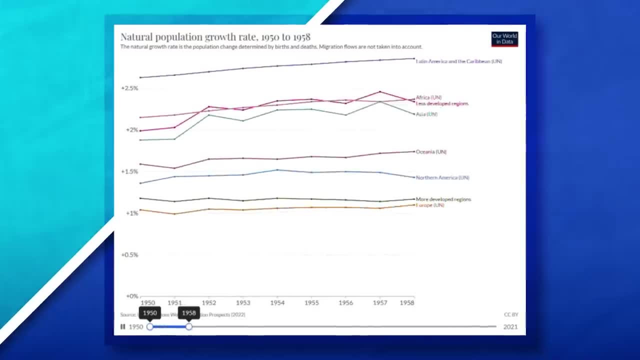 Notice that almost every country has constant urban growth. In fact, if we look at the different regions in Africa, we can see that every region is experiencing continued urban growth While, at the same time, birth rates are declining in core countries with more people looking 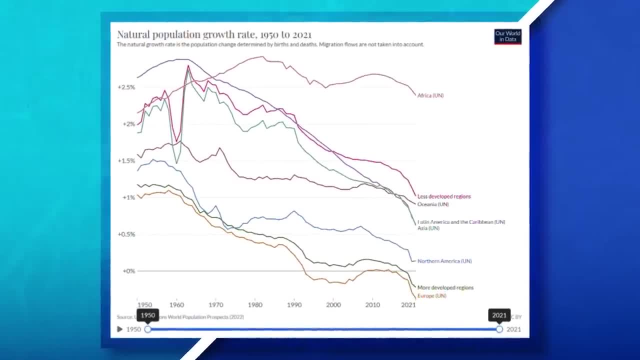 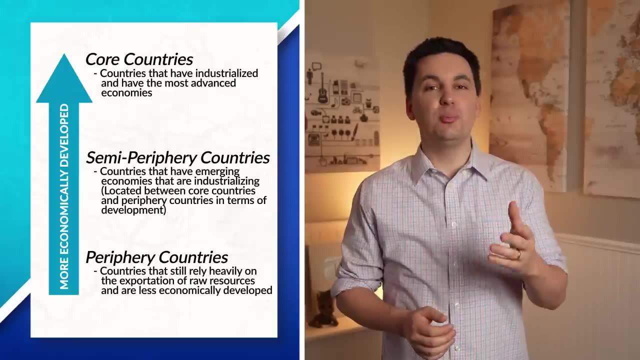 to live in suburbs and edge cities instead of densely populated areas. These demographic changes are just a few of the factors that are causing the future megacities and metacities to appear more in periphery and semi-periphery countries. As cities around the world experience population growth, they are likely to be more likely. 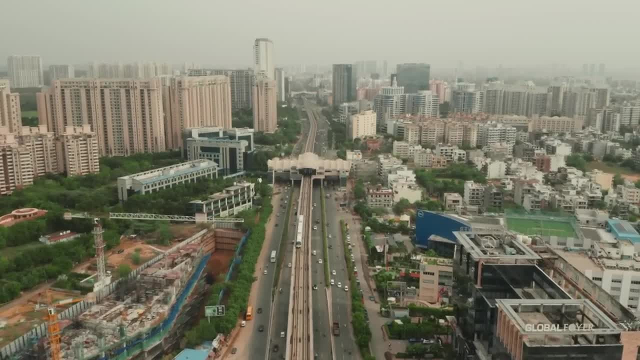 to experience population growth. As cities around the world experience population growth, they are likely to experience population growth. As cities around the world experience population growth, they will continue to be tested in new ways. More people in the city increases the demand for fresh water, housing, food and electricity. 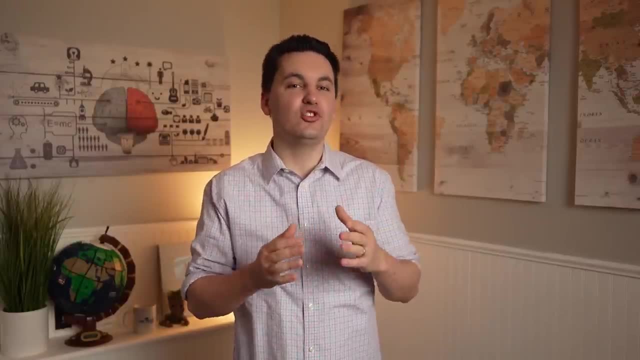 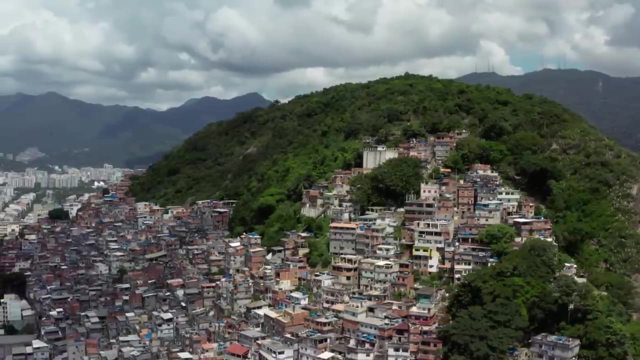 More people means more flushes and increased use of a city's sewer systems, roads and public transportation services And, unfortunately some cities and countries growth rates and urbanization rates are increasing at a rate that they simply can't keep up with. 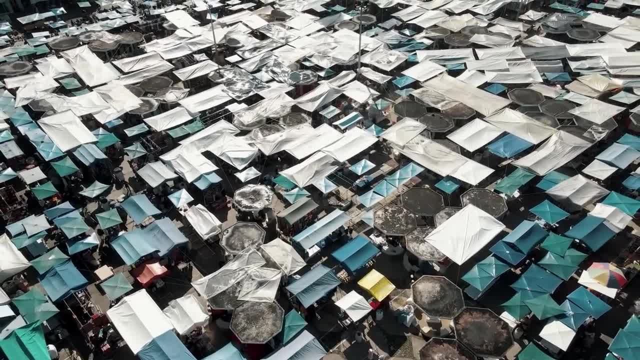 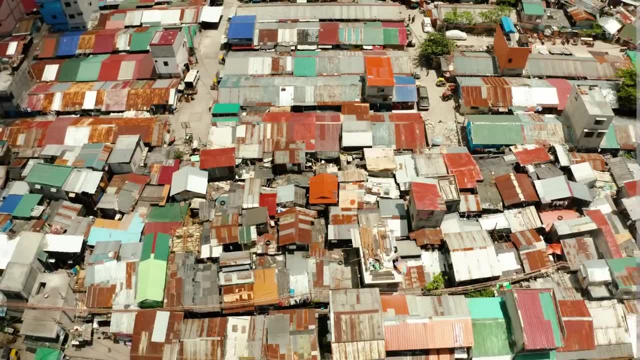 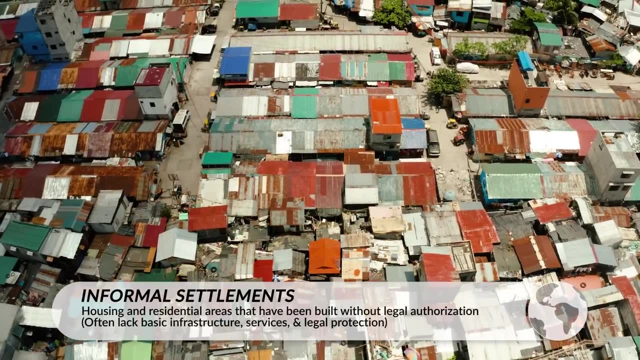 This has put new pressures on places which are struggling to keep up with the changing landscape has resulted in shortages and unequal distribution of different goods and services. For example, areas that struggle to provide enough affordable housing have seen the creation of informal settlements, sometimes referenced as favelas, squatter settlements or slums. 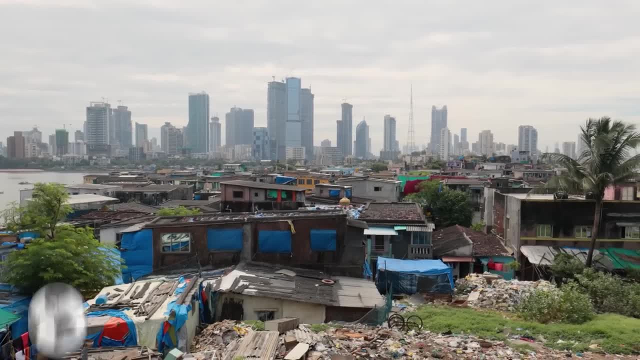 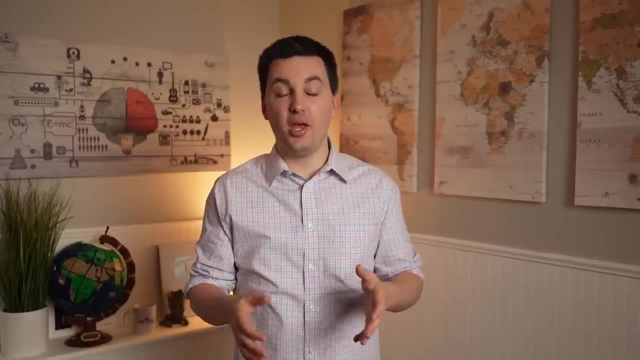 These areas often lack access to water, sewer systems and electricity Plus. to make matters worse, residents have no legal claim to the land and home they live in. We will go more into these concepts and other challenges cities face later in this unit. 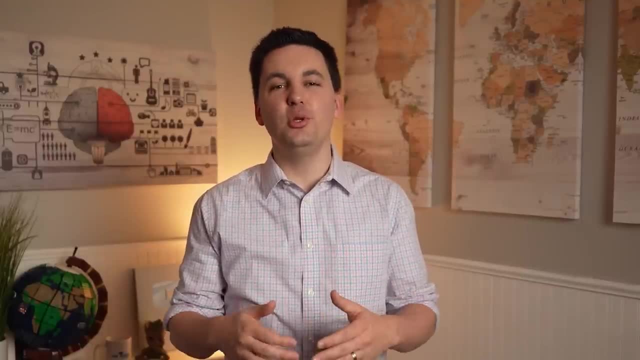 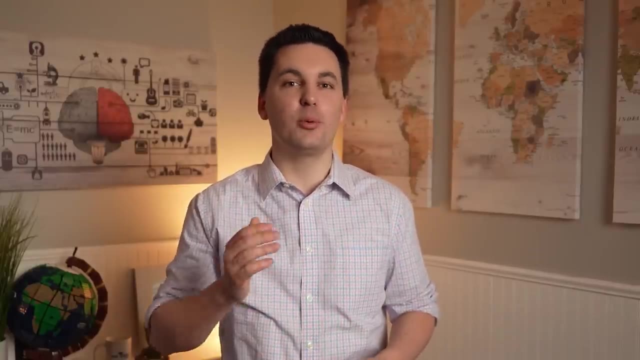 Now, while many periphery countries and semi-periphery countries are continuing to see increased rates of urbanization, many of the core countries are starting to experience counter-urbanization and suburbanation, Which is when people move from urban areas to settlements that are located around the 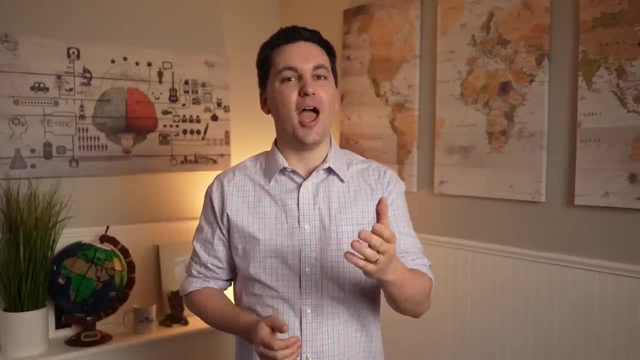 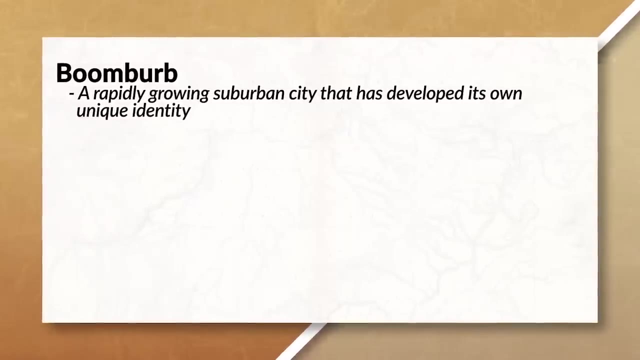 urban core, All of which has led to the rise of boomburbs, exurbs and edge cities. A boomburb is a suburban city that is rapidly growing. Often, these cities experience so much growth that they develop their own unique identity. 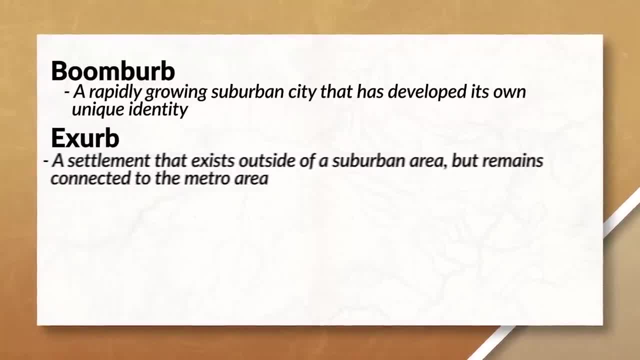 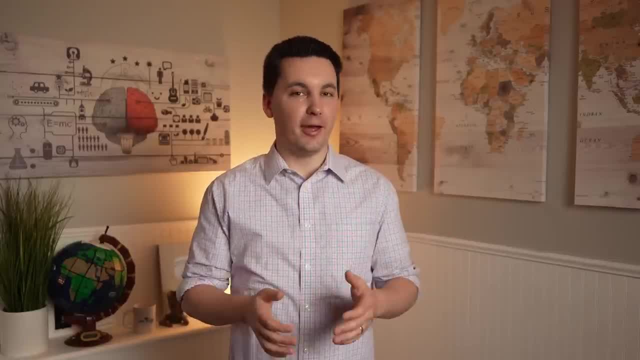 but still maintain that suburbanity. Exurbs, on the other hand, are settlements that exist outside of a suburban area but still remain connected to the larger metro area Oftentimes. individuals who live in an exurb will often get different goods and services. 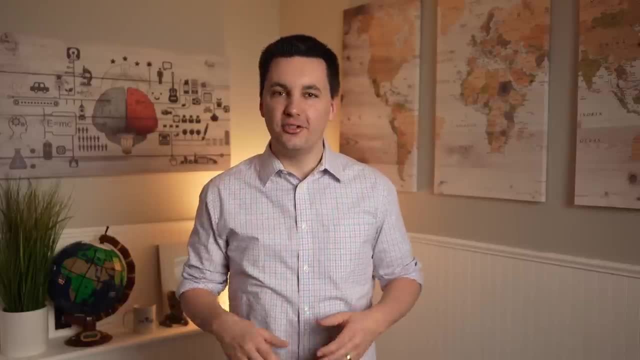 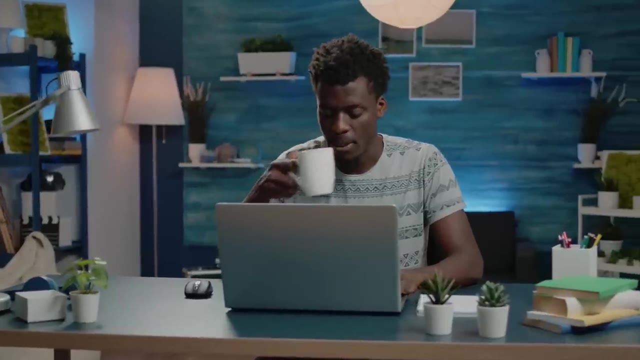 that they need from a nearby boomburb or edge city, instead of driving into a more densely populated urban area. Residents here also might decide to work from home, which, thanks to advancements in technology and communication, is continuing to happen more frequently in settlements around the. 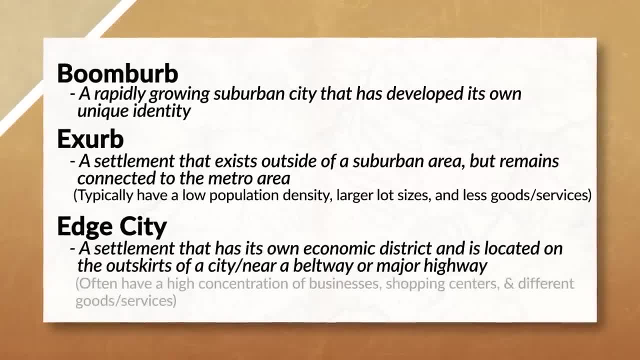 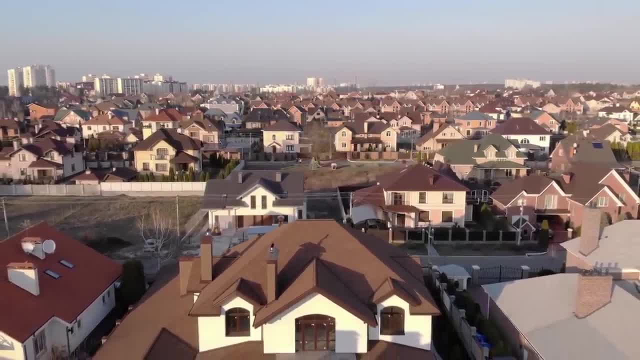 world. Now I mentioned edge cities. They are settlements that have their own economic district and are located on the outskirts of a city. Traditionally, these cities have a lower density, with homes and businesses being more spaced out. They are connected to a major roadway or beltway, which are highways that surround an urban. 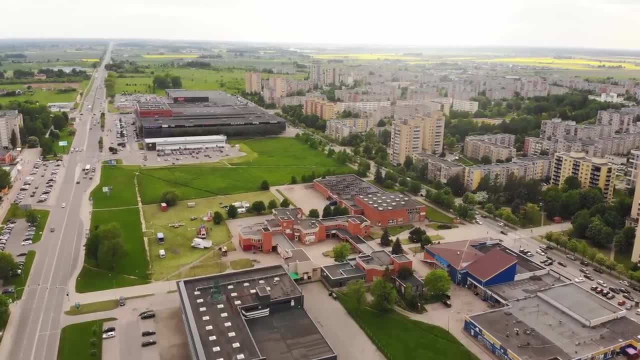 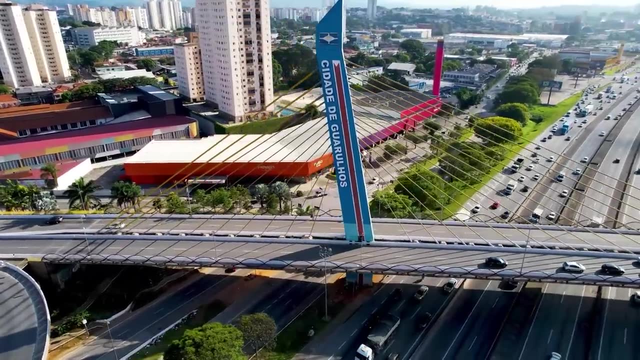 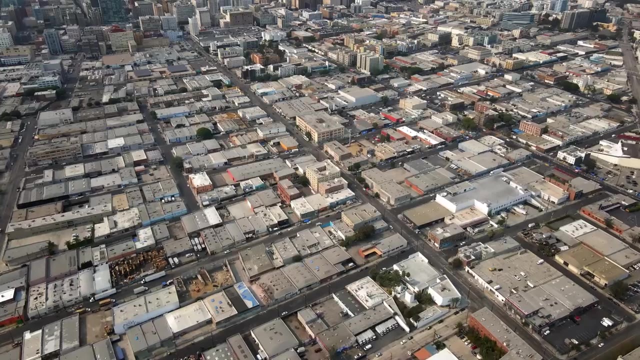 area. This allows people to quickly travel between different edge cities and to access the different goods and services that each city offers. Edge cities often have their own shopping malls, different retail stores, restaurants and medical services. This leads to people, businesses and goods and services to locate outside of the core. 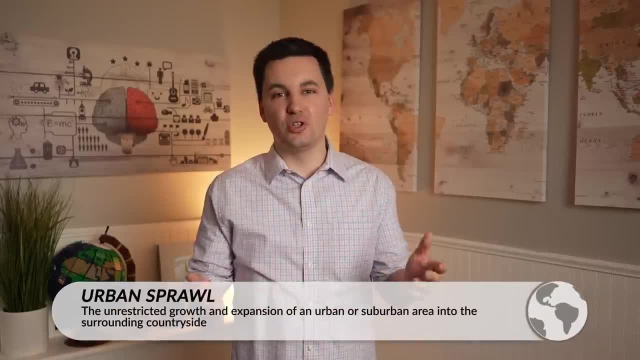 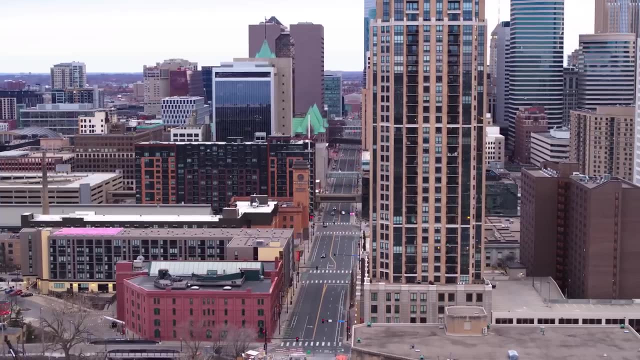 urban area. It's known as urban sprawl. When looking at the spatial layout of these different settlements, we can often see a central business district at the center. As sprawl continues to happen, we see urban decentralization occur, which is when people 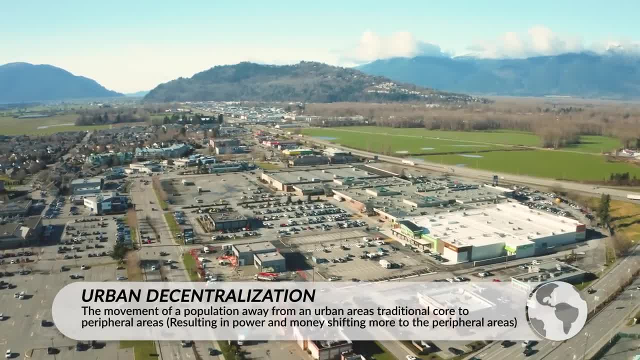 and businesses move away from the urban core and toward settlements in the outskirts of the city. This results in certain powers and responsibilities to transfer from the urban core and go to these new cities. This is where urban sprawl is going to happen. It's a central business district. 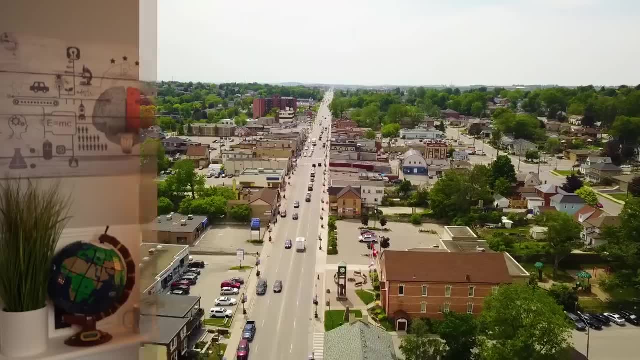 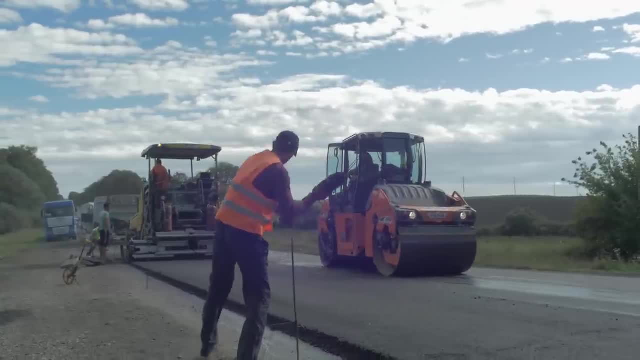 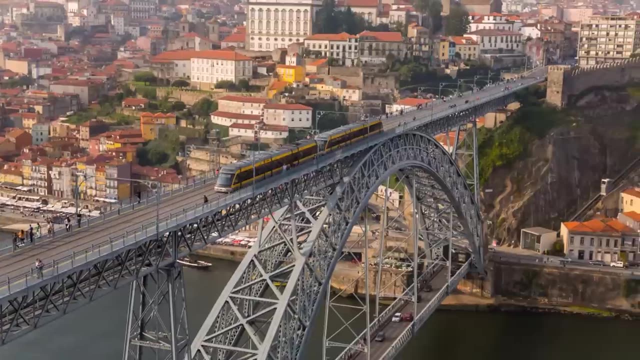 As time goes on, we'll continue to see more roadways created and public transportation expand, All of which will lead to new edge cities and boom burbs to pop up outside of core urban areas. Since people can now quickly go in and out of the urban area, new roadways often connect. 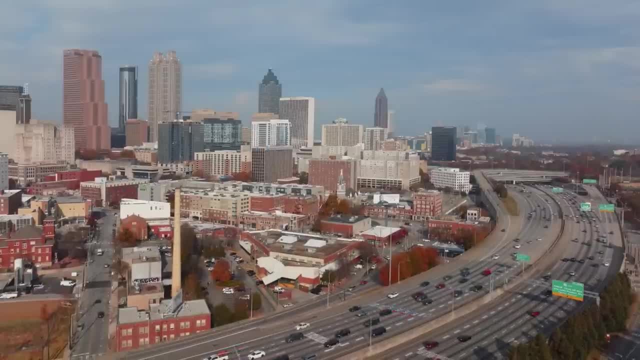 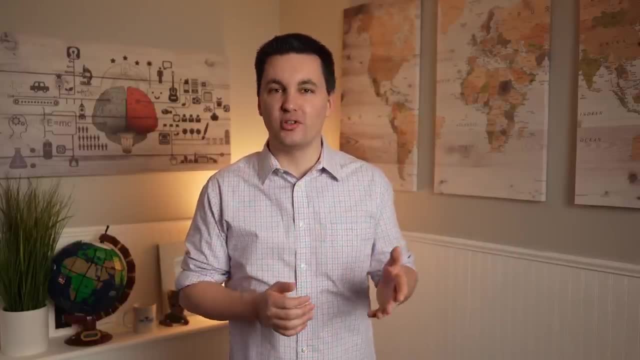 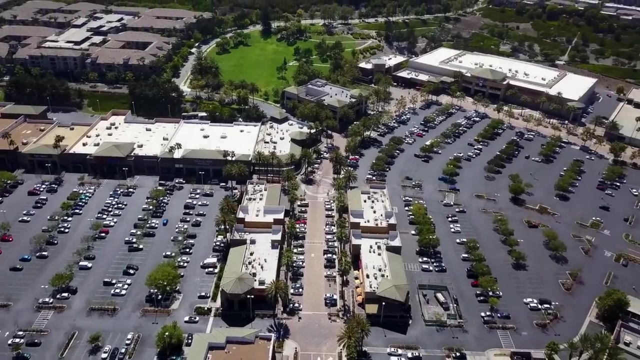 to interstate systems and beltways which not only connect to the CBD but to other edge cities and settlements as well. This makes it easy for people to not only quickly get in and out of the central business district, But access different goods and services from surrounding settlement. now, instead of having to go into the city, people can get what they need. 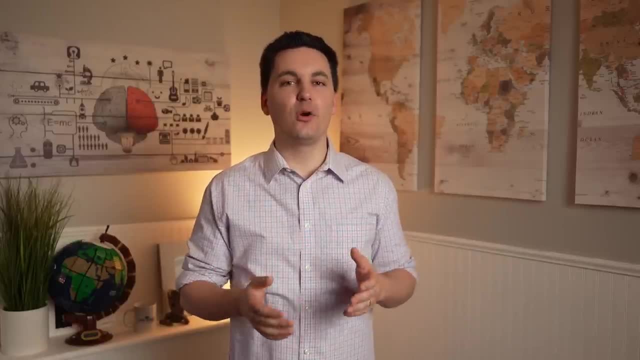 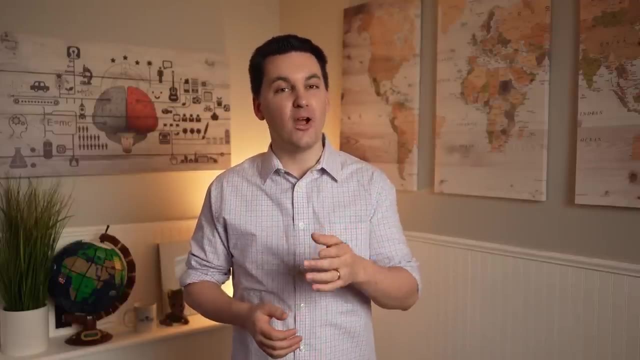 quicker and more efficient. oftentimes, people will interact more frequently with nearby edge cities or Boom burbs instead of going into the central business district because it's closer and faster. now, speaking of different settlements and their locations, We can also see the bid-rent theory at play, a concept 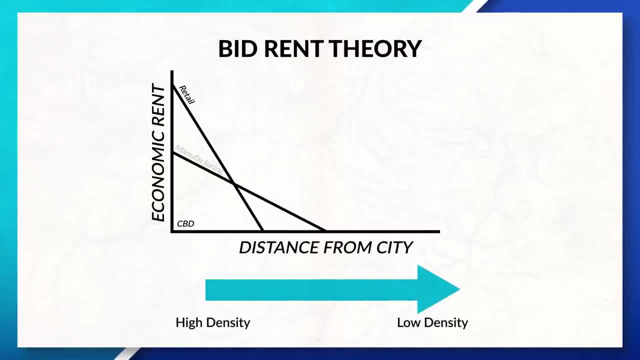 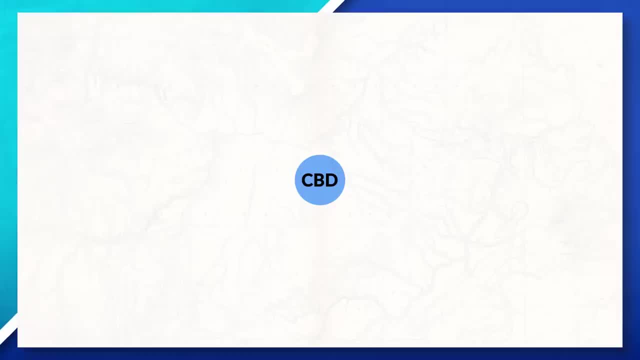 We last talked about in our unit 5 video. We can see that as you move farther away from the central business district, the cheaper the land gets, Which impacts the spatial layouts of settlement. places that are closer to the central business district often see more buildings close together. 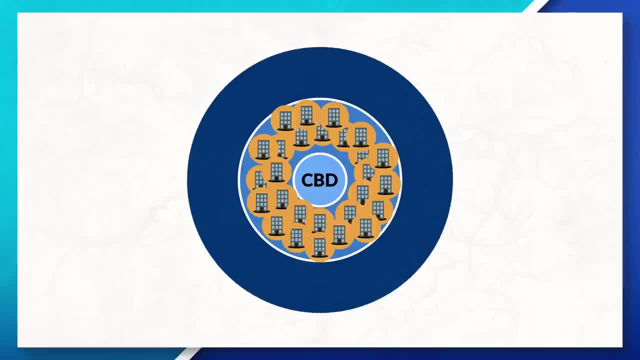 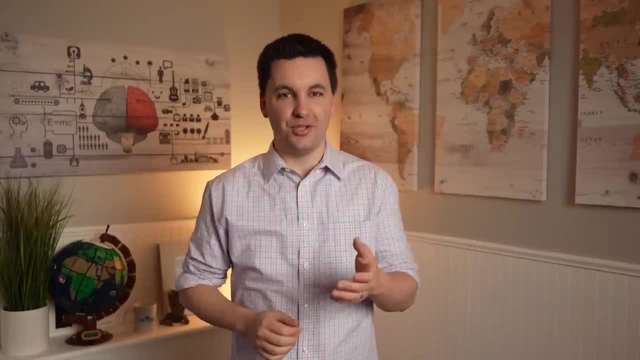 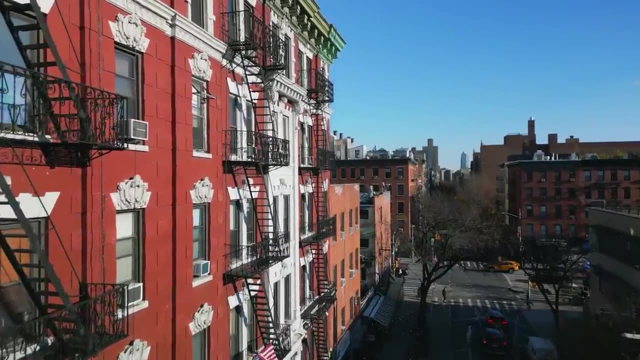 With expansion happening upward, while places that are farther away from the CBD often expand Horizontally and are more dispersed. homes that are located farther away from a central business district Often have a front yard And a backyard and access to more green spaces, while homes that are near or in the CBD 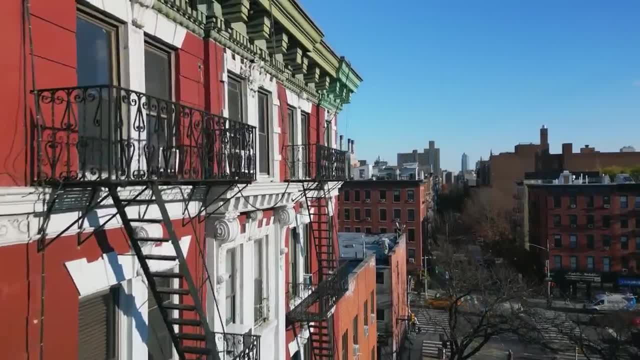 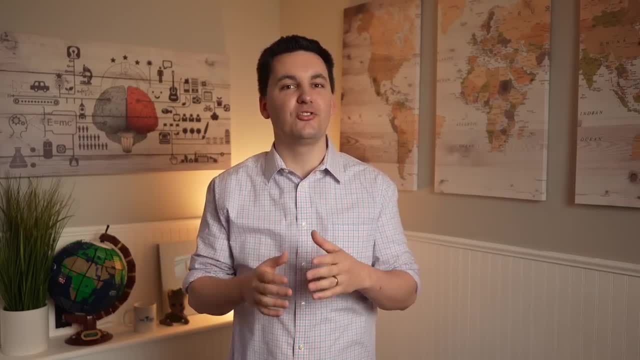 Often do not have space to expand outwards and are more likely to be built on top of one another. all of this is because of the cost and the availability of land changing as our population density changes. now, as we continue to see more advancements in technology, transportation and 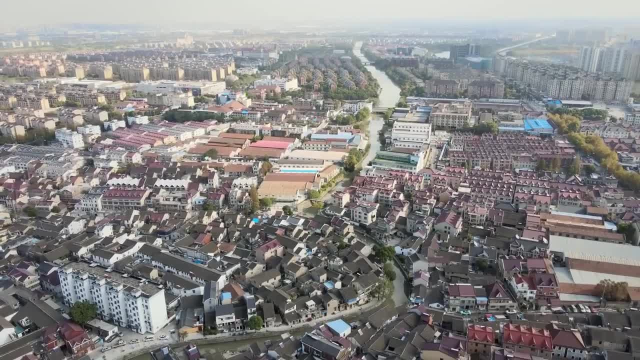 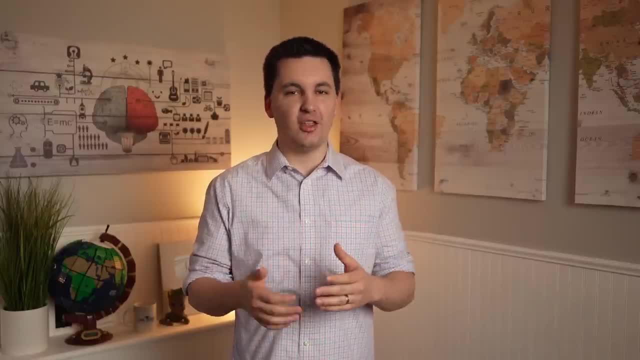 Communication. we will continue to see more people move to the suburbs, Which will also lead to businesses and public services to move as well. So we can see that the growth of cities and the challenges that they face will vary across different Geographic location and will continue to change over time. today, 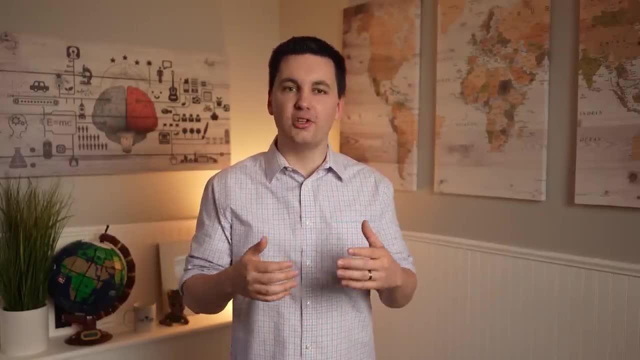 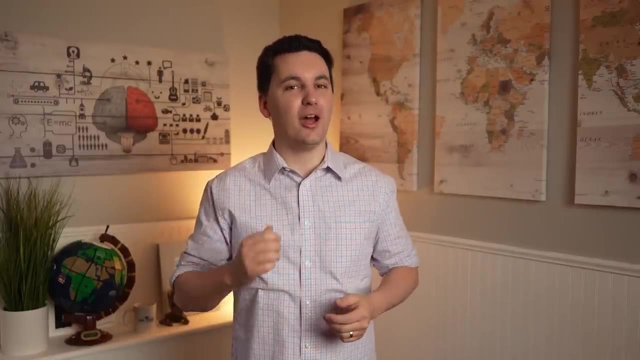 We can see that countries in the periphery and semi-periphery are more likely to have high rates of urbanization, While core countries are starting to see a shift and a rise in suburbanation and counter urbanization. All right, now comes the time to practice what we have learned. 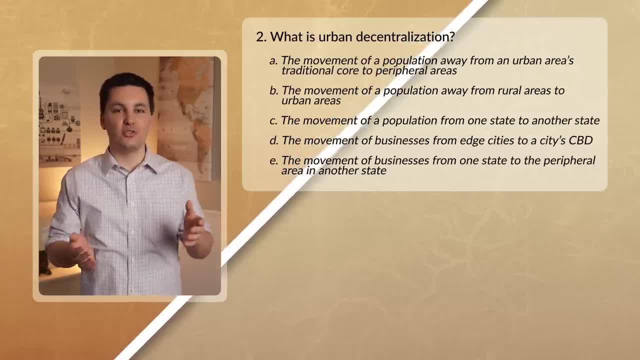 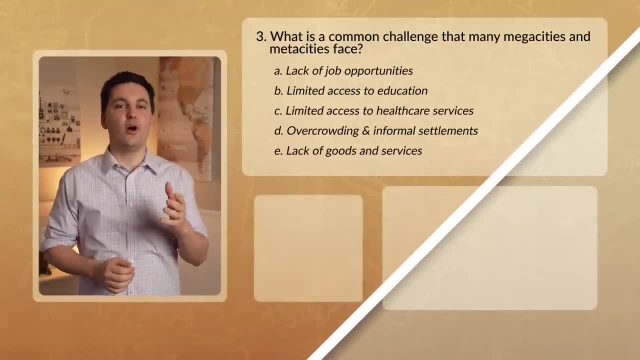 Answer the questions on the screen and when you are done, check your answers down in the comment section below. and while you're down there, Don't forget to hit that subscribe button If you found value in the video and check out my ultimate review packet for more help with everything ap human geography related.